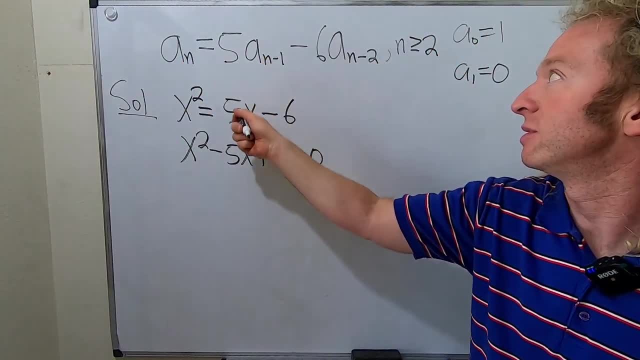 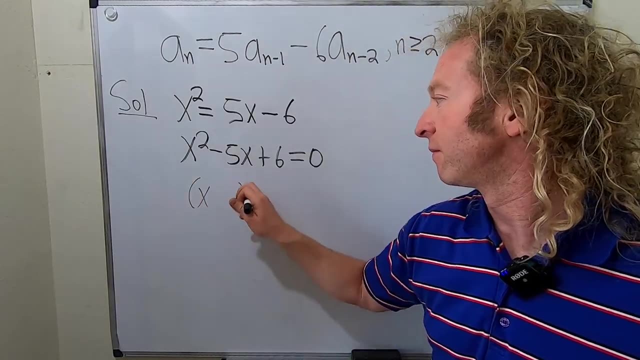 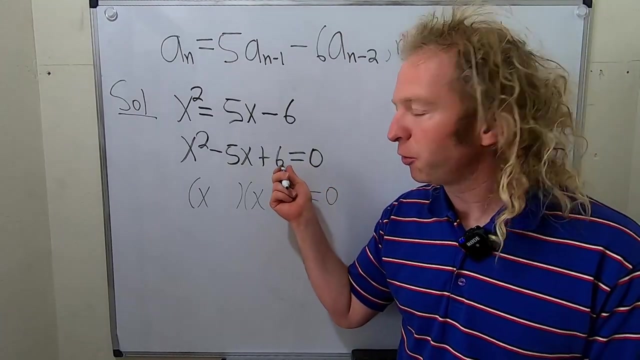 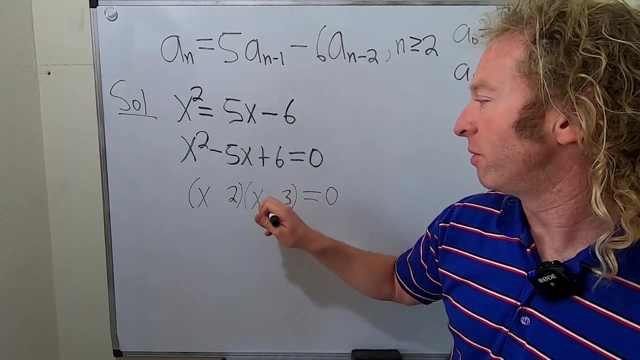 just memorize it right: A sub n turns into that, that turns into that. that's always a constant, every single time. Let's try to factor this and solve for x. And again, this is called the characteristic equation, It's also called the auxiliary equation. We need two numbers that multiply to six but add to negative five. I think two and three should work. So two and three, And these are both minus signs because they need to add to a negative 5x. So you get x minus two. 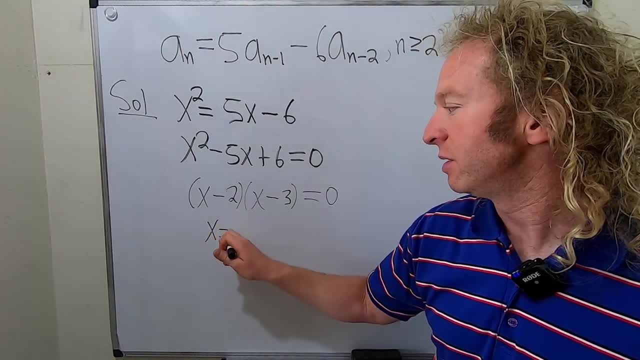 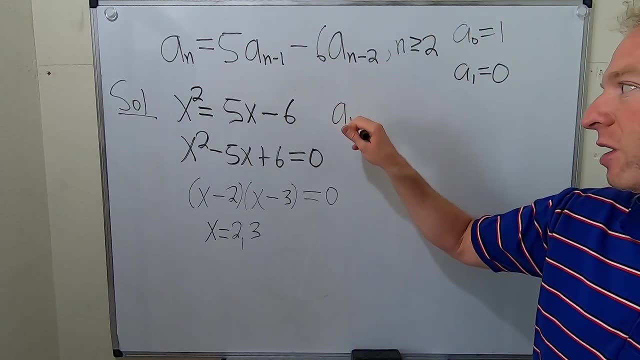 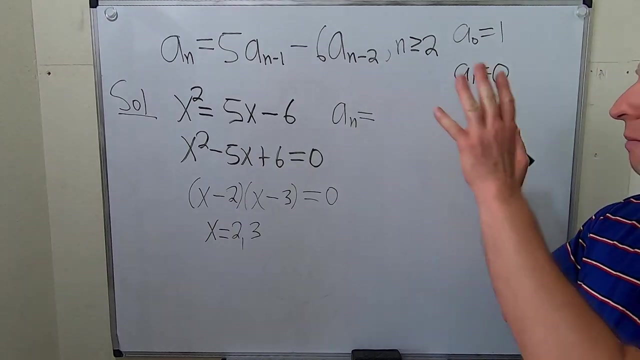 equals zero. or x minus three equals zero. So we have two distinct real roots. So whenever you have two distinct real roots, the answer has the following form: right, You just go straight to the answer. So I need a constant here. So, again, depending on the book, depending on your teacher, if you have a teacher, they use different constants. I'm going to use C. okay, I'm going to use big C one times two to the n, plus big C two times three to the n. So it's always that. 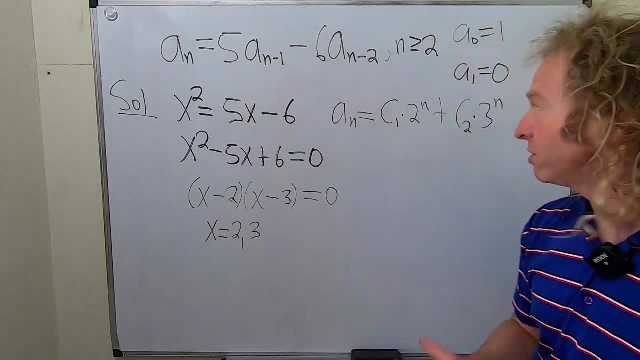 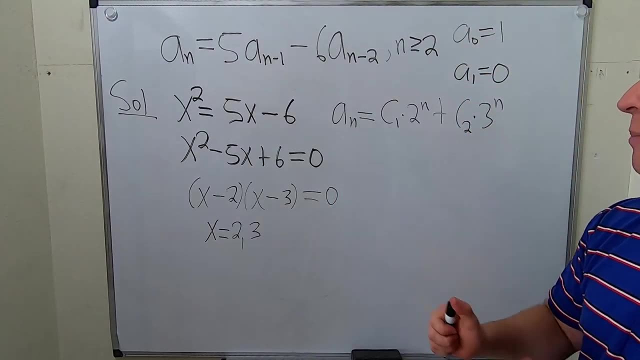 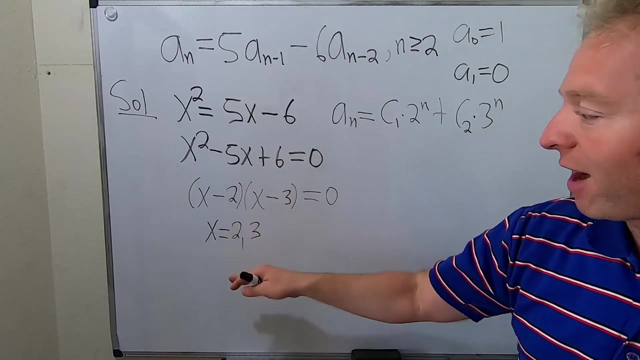 it's always if they're different. So if you get distinct real numbers, that is the form of the solution, right? So this is the distinct real roots case Recap. you see this. you change this to a two. that's an x, that's a constant. set it equal to zero. okay, Factor. get the answers If. 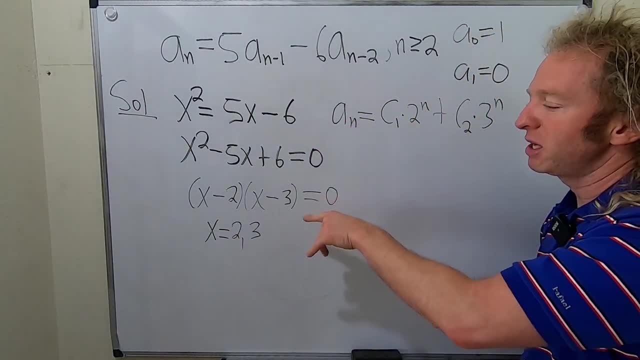 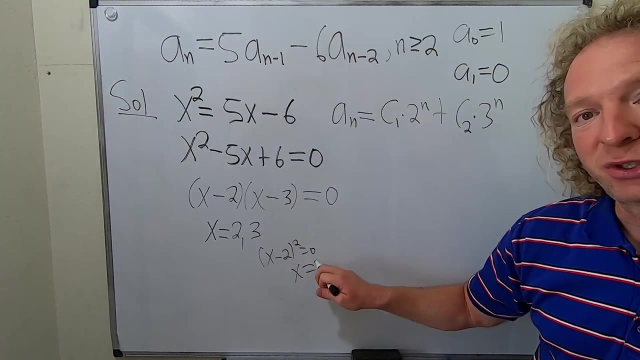 they're different numbers. that's the answer. If you get a repeated number like say it was just like two And like say it was this x minus two squared equals zero, then you would get x equals two. that's a repeated root of multiple C two. it would be the same, except you would have C one. 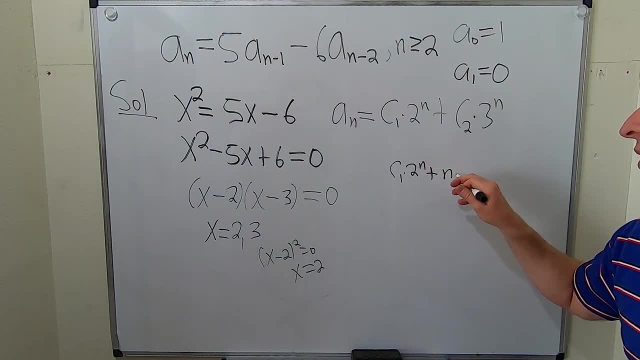 two to the n And since it's repeated, you would put an n there, okay, So it would be C two and two to the n. So whenever you have repetition, that's what you do If you've taken or if you know. 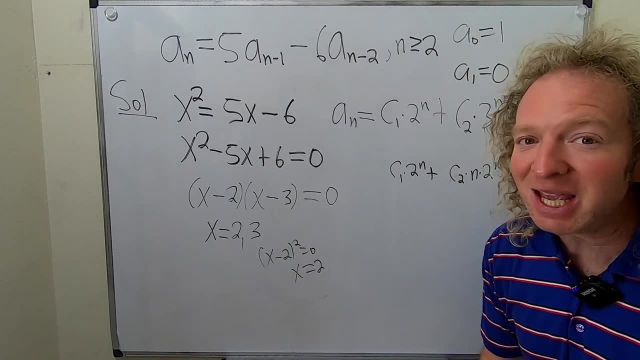 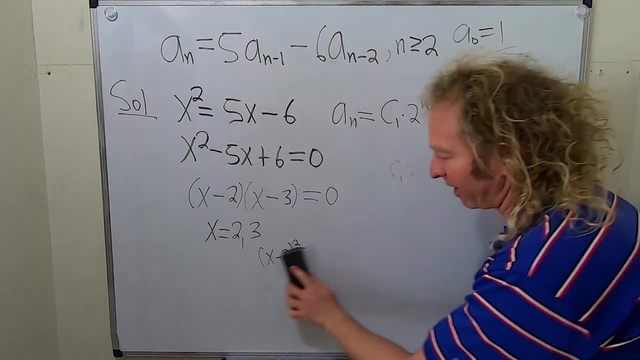 something about differential equations. this is exactly the same as when you solve the higher order linear, homogeneous differential equations. If you haven't, don't worry about it, But it's the same thing. It's one of those things where you learn some math and then you can apply it. 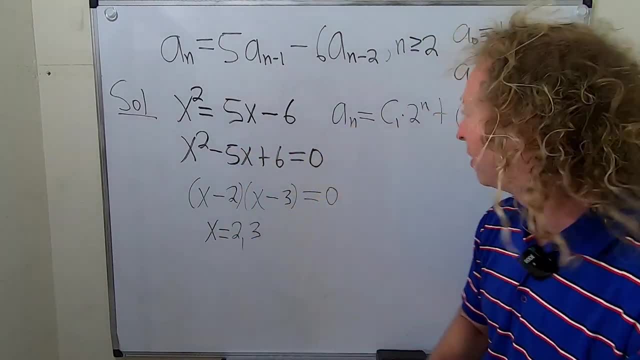 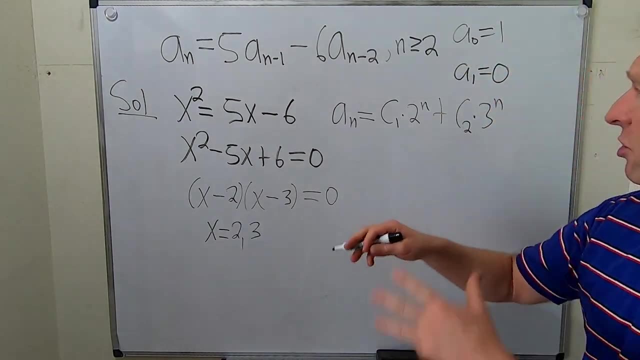 somewhere else. So this is something that doesn't just appear here. All right, so that's the answer. Now we just have to use our initial conditions to find the C's, and then we're done. Okay, so let's impose our initial conditions. I'm just going to draw a line here for a division of 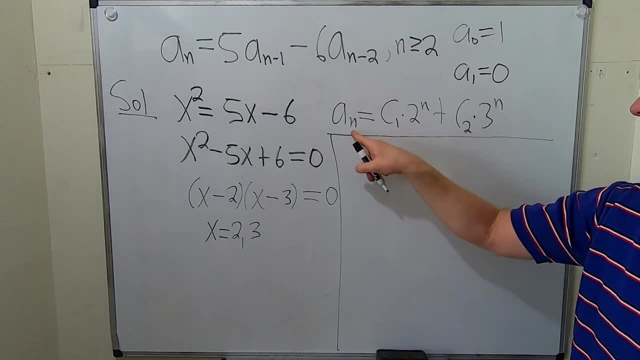 thought So, using this one we'll have- I'll put a one here, because that's one- and then n is zero, So it's just C one. three to the zero is one, So it's just C two. Very good, Now let's use this. 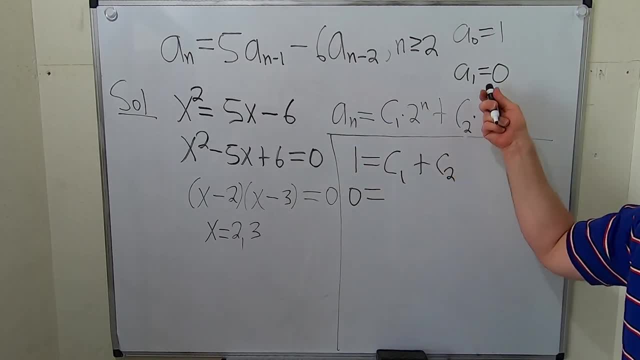 one, So I'll put a zero here. And then n is one, this time right. So n is one, So it'll be C one times two plus C two, and then n is one, So it's times three. Let me check my work, because I have. 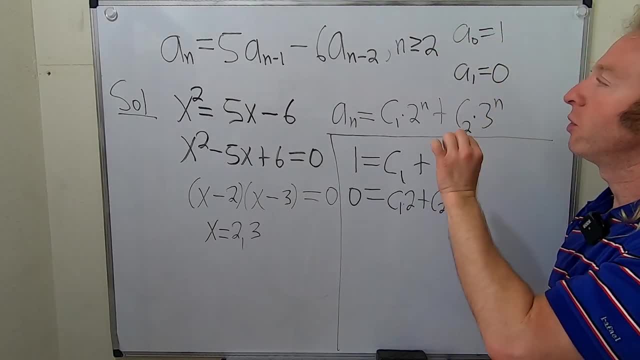 not done this problem. So a sub zero is equal to one, So we put the one here. Okay, it looks okay. And then we said n was zero, right? So two, three, four, five, six, seven, eight, nine, ten, ten. 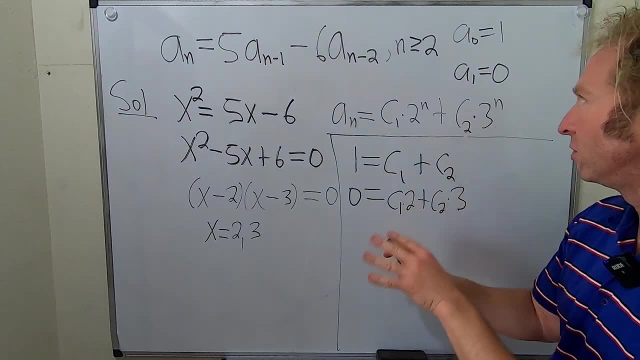 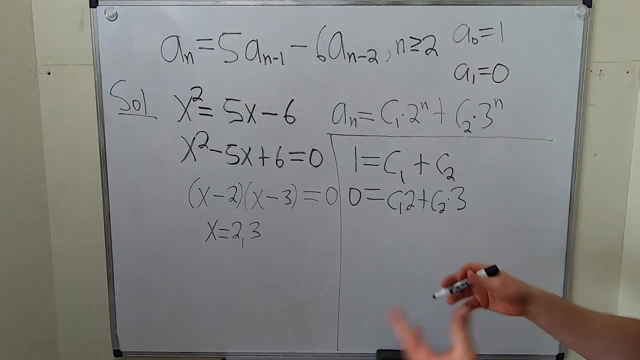 two to the zero is one Boom. three to the zero is one Boom. everything looks good. A sub one is zero, Ah, good stuff. Two to the: it looks good, It looks really good. We have to solve this. 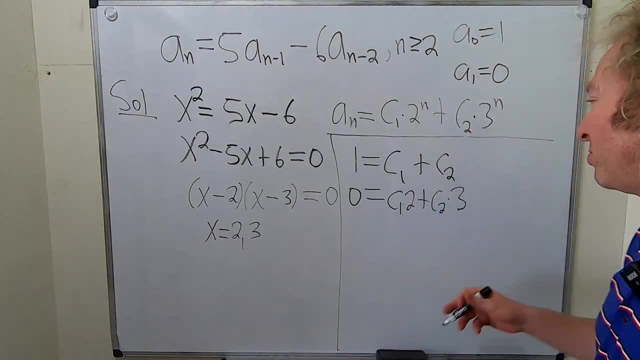 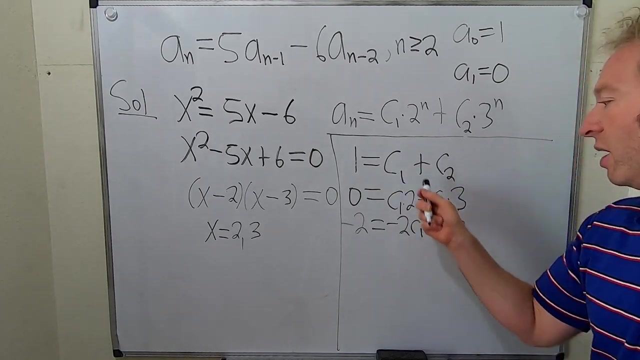 equation. I love the elimination method. I don't like substitution, I'm it's. everyone has their thing. I'm going to multiply this by negative two, So we get negative two C one minus two C two. And the reason I did that right is multiply the first equation by negative two is so that now 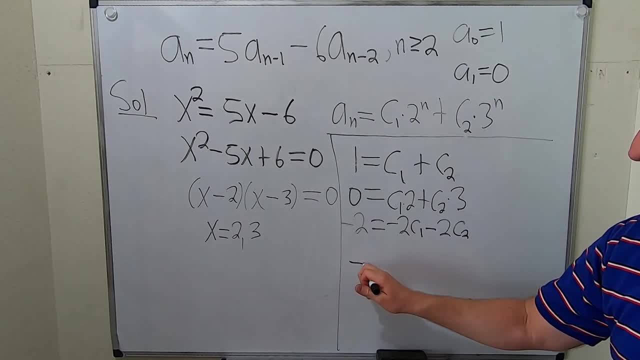 when you add these, you're going to get negative two C one minus two C two. So you're going to cancel the C ones, right? So this is going to be negative two equals. you add these up, it goes away. This looks really weird. but three C two minus two C two is simply C two. Yeah, Oh, that's. 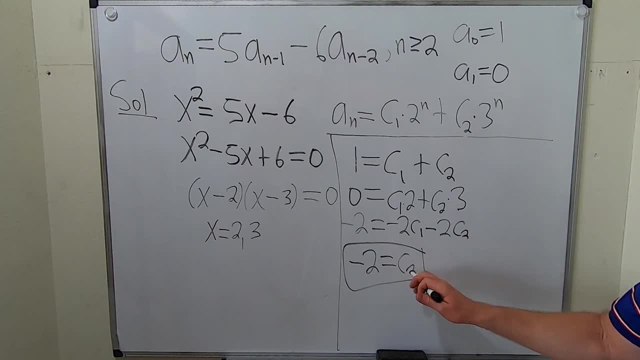 how you do it right. We've got one of them, So now you take this one and plug it in here. Let's see. So we get one equals C one minus two, right, Minus two, because C two is minus two. So I put.